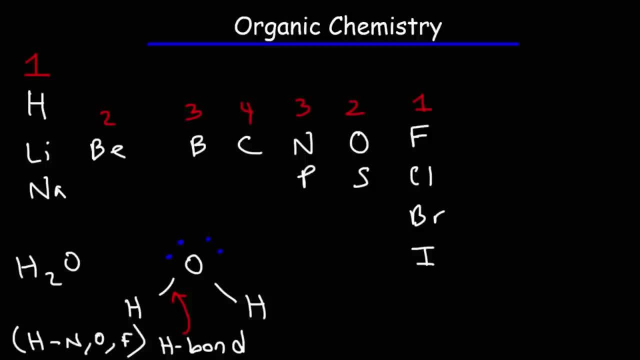 oxygen or fluorine. Hydrogen bonding explains why water has such a high boiling point. Now let's say, if we have methyl fluoride, How can we draw the Lewis structure for that molecule? So we know that carbon likes to form four bonds, so we're going to put that in the middle. Hydrogen likes. 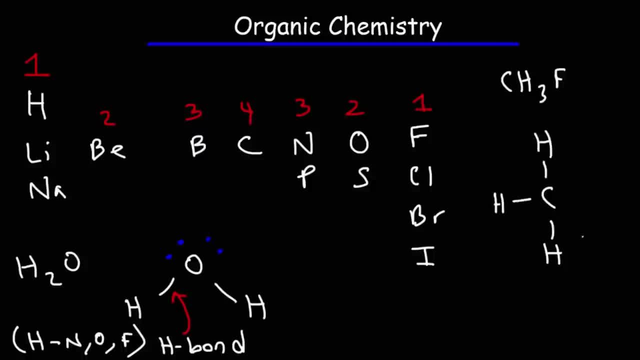 to form one bond. Fluorine also likes to form one bond, so this is the best Lewis structure that we can make And if you want, you can add three lone pairs to fluorine so that it has eight electrons around it. Elements in the second row, like carbon, nitrogen, oxygen and fluorine. they like to have eight electrons. 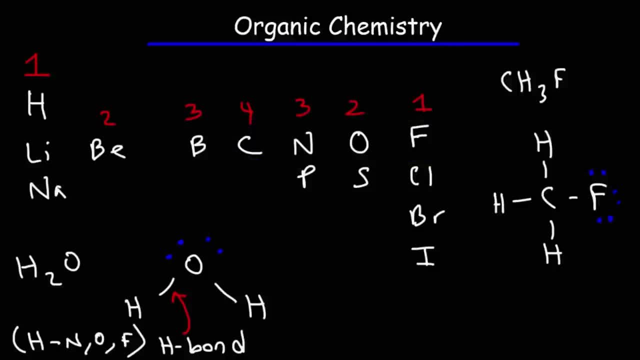 They don't always have to have eight, but ideally speaking they like to have eight so that they can be stable. But that's the structure of methyl fluoride. Now, the carbon-fluorine bond is a polar bond. Carbon has an electronegativity value of 2.5, and the electronegativity value of fluorine is 4.0. 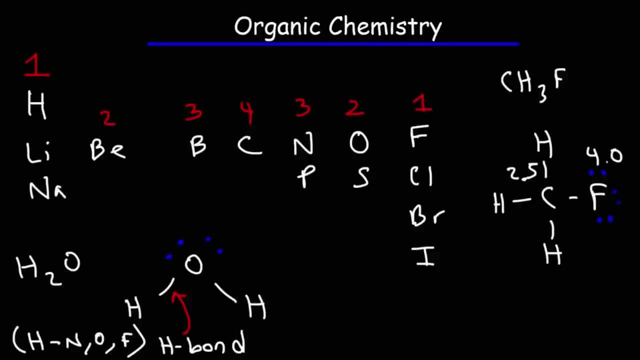 Whenever the electronegativity difference between two elements is 0.5 or more, the bond is sent to be polar. So this is a polar bond. It's not a hydrogen bond, because fluorine is not directly attached to hydrogen, but it's a polar covalent bond. 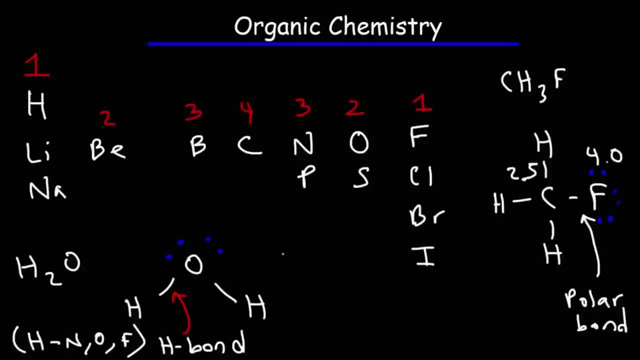 Now you might be wondering: what does it mean for a bond to be polar? A polarized object is an object that is neutral overall but has charge separation, That is, one side is positive and the other side is negative. So this is a polarized object. 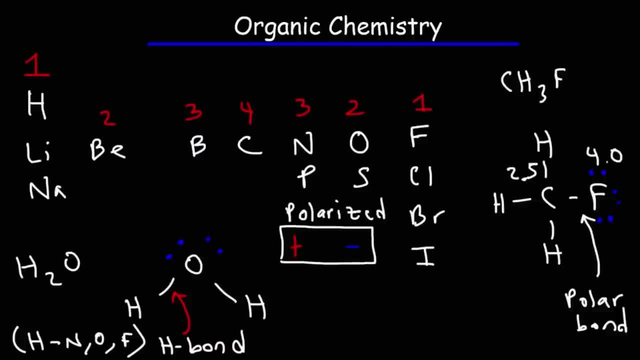 The bond is polar because fluorine carries a partial negative charge due to the fact that it's more electronegative than carbon, So it pulls electrons. The bond pulls electrons toward itself and carbon, being less electronegative, has a partial positive charge. 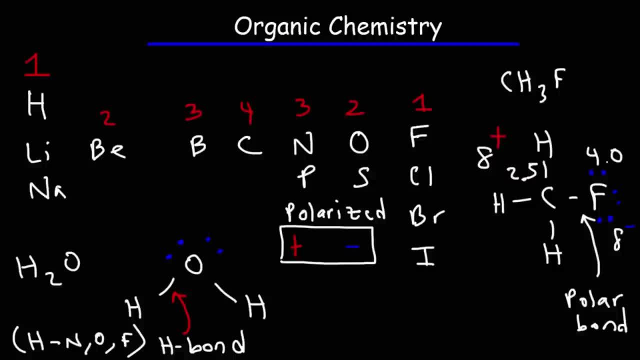 So due to that charge separation, we can say that the carbon-fluorine bond is polar, Now the carbon-hydrogen bond, that's a nonpolar bond. The reason being is the electronegativity difference between carbon and hydrogen is less than 0.5.. 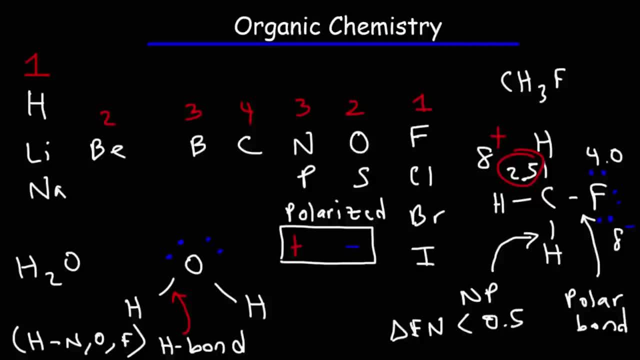 Carbon, we said its electronegativity value is 2.0.. Hydrogen is 2.1.. So the difference between the two is 0.4.. So understand this. anytime you see a hydrocarbon or a bond that contains carbon and hydrogen, those bonds are nonpolar bonds. 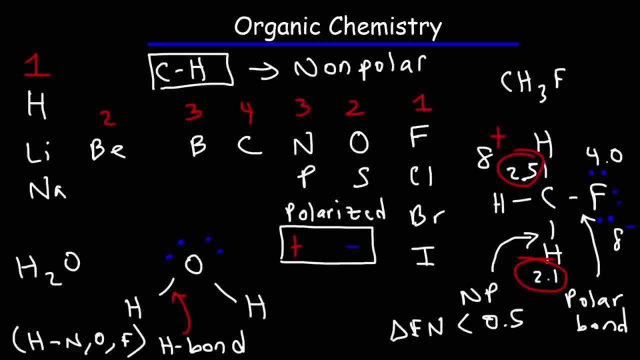 Because sometimes you need to determine if a molecule is polar or nonpolar. So, for instance, methane CH4, that's a nonpolar molecule because it only contains carbon and hydrogen. So far we've considered two types of covalent bonds. 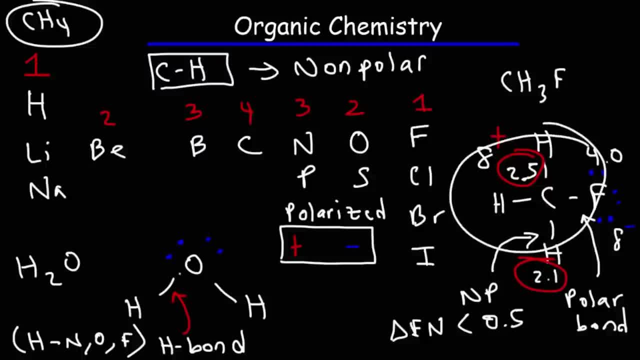 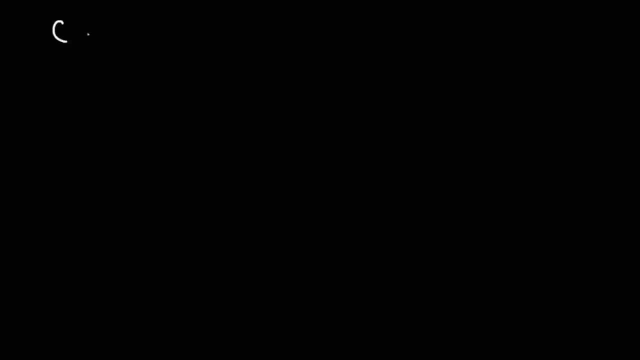 Polar covalent bonds and another special type, which are hydrogen bonds, And we also talked about nonpolar covalent bonds, like the carbon-hydrogen bond. That's a nonpolar covalent bond, But you need to understand the difference between a covalent bond and an ionic bond. 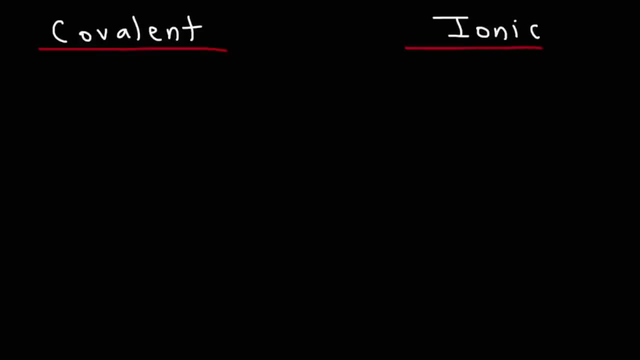 In a covalent bond, the electrons are being shared. They can be shared equally or unequally. So in the case of the hydrogen molecule H2, the electrons in this bond are being shared equally between these two atoms, Because the atoms are identical. 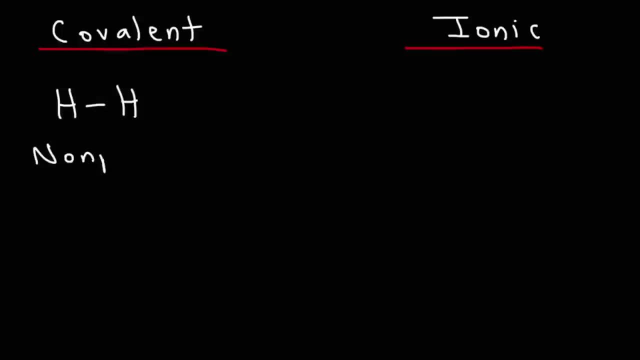 So that's known as a nonpolar covalent bond, which I put CB for covalent bond. In the case of hydrogen fluoride, that is a polar covalent bond. Hydrogen has an electronegativity of 2.1. 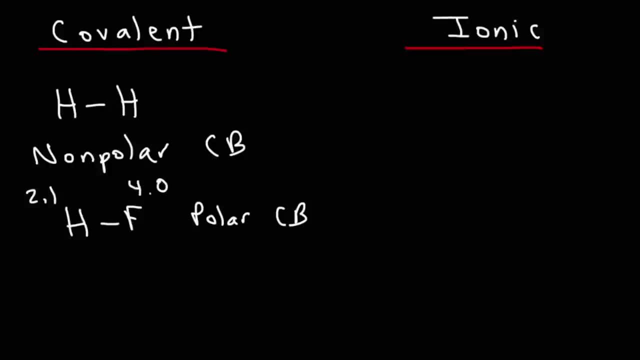 Fluorine has a value of 4.0.. So hydrogen is going to be partially positive, Fluorine will be partially negative And this is a special type of polar covalent bond That's a hydrogen bond. So those are some two examples of covalent bonds. 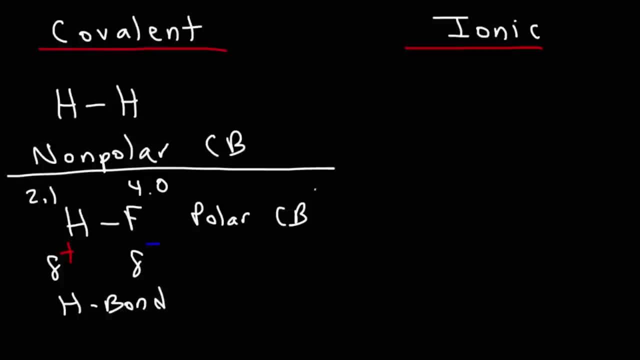 You have nonpolar covalent bonds And polar covalent bonds, So make sure you understand the difference. here The electrons are shared equally. That's the key word, And in this case, the electrons are shared unequally. 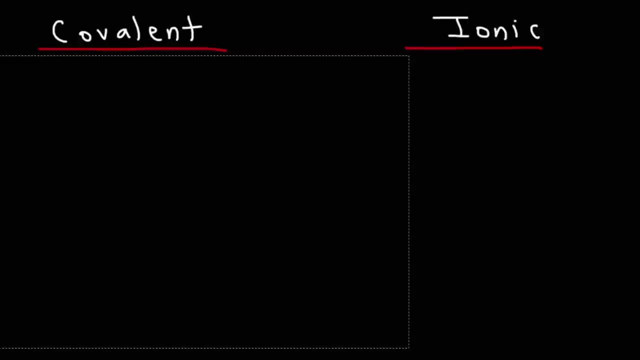 Fluorine is going to have a tighter hold on those electrons. Now let's talk about ionic bonds. So in an ionic bond the electrons are not shared, They're transferred. A good example is the reaction between sodium metal and chlorine. 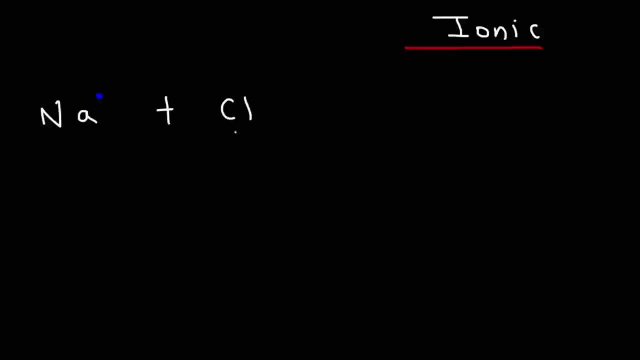 Sodium has one valence electron. Chlorine has seven. Sodium is a metal And chlorine is a nonmetal. Metals like to give away their electrons Because they're electropositive. Nonmetals like to accept or acquire electrons Because they're electronegative. 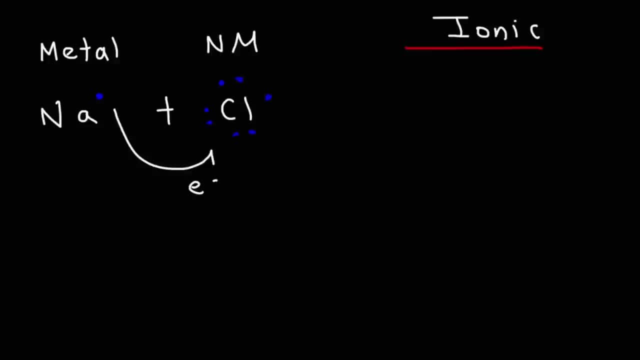 So sodium is going to give one electron to chlorine. A half arrow represents the flow of one electron, A full arrow represents the flow of two electrons. So in this reaction sodium is going to turn into the sodium plus ion Which is known as a cation. 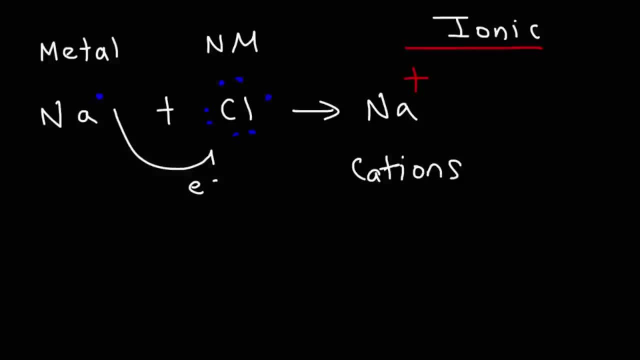 Positively charged ions are called cations, Now chlorine. when it acquires an electron it becomes chloride, So now it has eight electrons. It's going to now have a negative charge. Negatively charged ions are known as anions. 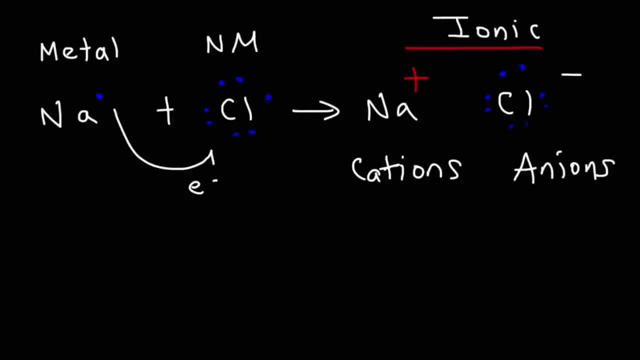 Now, going back to physics, you know that opposite charges attract one another. So a positively charged ion will feel a force of attraction to a negative charge. So these two charges, they attract to each other. And that force of attraction, that electrostatic force, is what keeps the ions in an ionic crystal together. 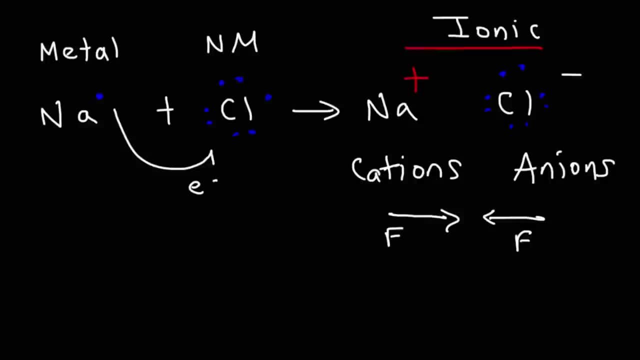 So that creates that ionic bond, That electrostatic force of attraction that pulls the sodium and the chloride ions together. So now you know the difference between an ionic bond and a covalent bond. So now we're going to spend some time drawing Lewis structures of certain organic compounds. 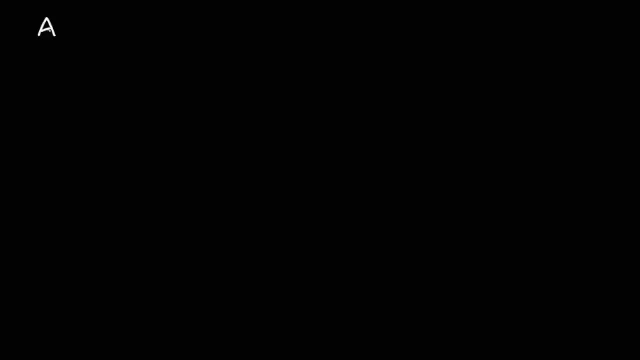 But before we do, let's talk about some common names of alkanes. Alkanes are saturated organic compounds, Meaning that the carbon atoms are filled with hydrogen atoms. Methane is a one carbon alkane: It's M-E-T-H-A-N-E. 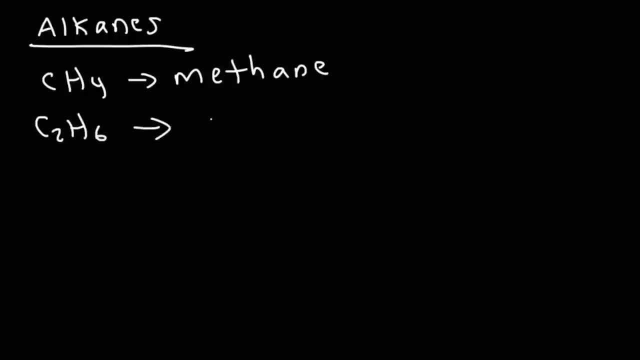 A two carbon alkane: C2H6.. This is known as ethane, C3H8.. This is called propane, C4H10.. This is known as butane. So alkanes generally follow this formula: CnH2n plus 2.. 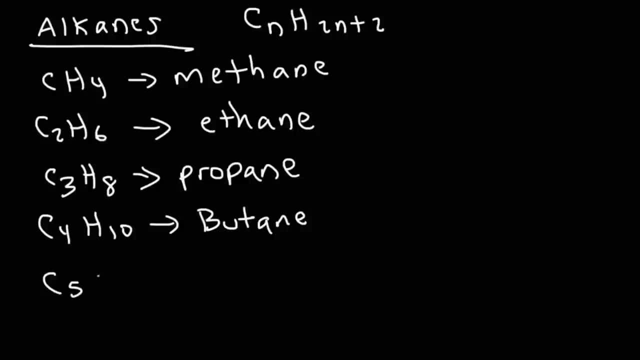 So a five carbon alkane will have 12 hydrogen atoms. If n is 5, then it's going to be H2 times 5 plus 2.. So that's 10 plus 2, you get 12.. A five carbon alkane is known as pentane. 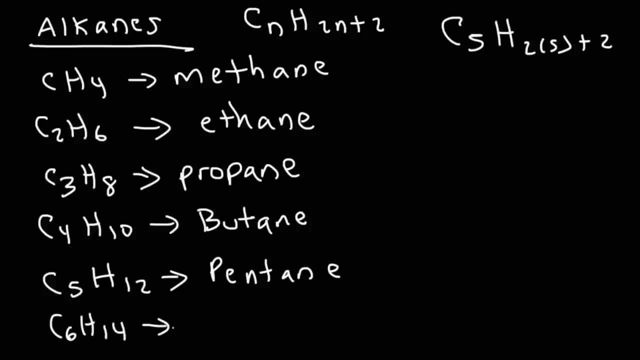 A six carbon alkane is known as hexane. You may want to take some notes, by the way, Because you'll need to know this, at least up to 10.. The seven carbon alkane, that's heptane. Next we have octane. 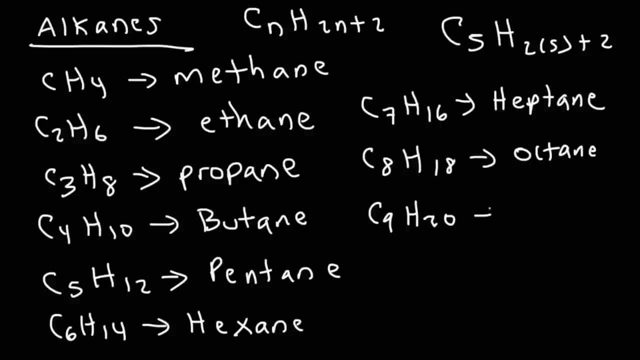 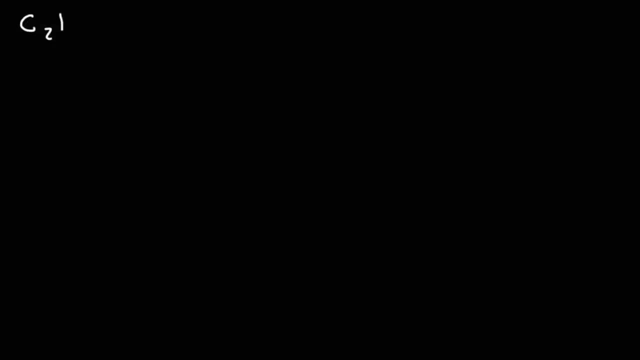 And then after that, this is, that's a 20. This is nonane, Or, if you want to call it nonane, And then C10H22, that's known as decane. Now let's talk about how to draw the Lewis structure of C2H6. 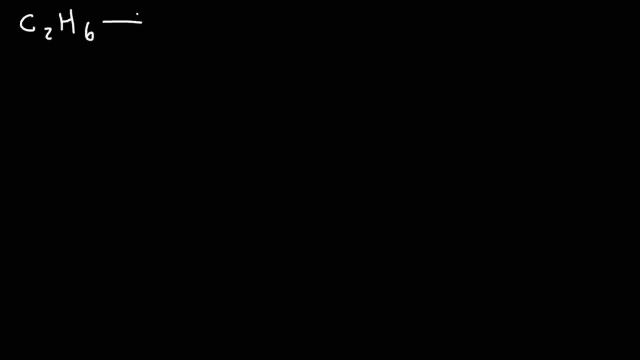 C2H6, we know that's ethane And you can write the condensed structure like this: It's CH3CH3.. So this tells you how many hydrogen atoms are on each carbon. The first carbon has three hydrogen atoms And that's attached to the second carbon. 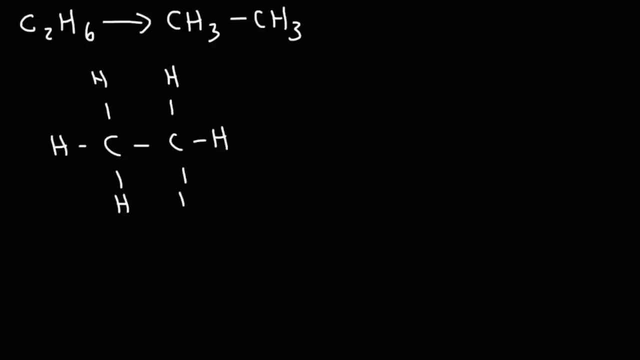 which also has three hydrogen atoms. So that's how you can draw the Lewis structure of ethane. Now what about C2H4?? How would you draw the Lewis structure for that? So this time, each carbon atom is going to have two hydrogen atoms instead of three. 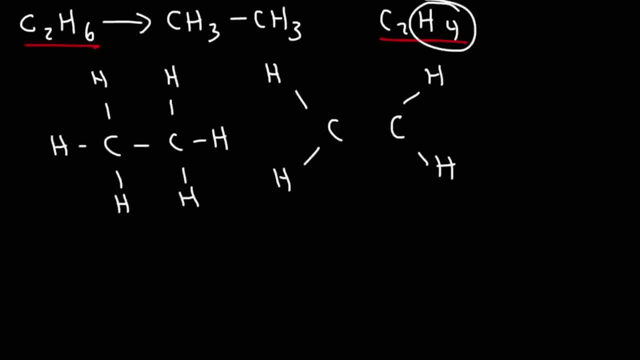 Because there's a total of four And you want to make sure that the four hydrogen atoms are distributed equally. So what bond do we need between the two carbon atoms? Well, we know that carbon likes to form four bonds, So the only way this is going to happen is if we put a double bond between the two carbon atoms. 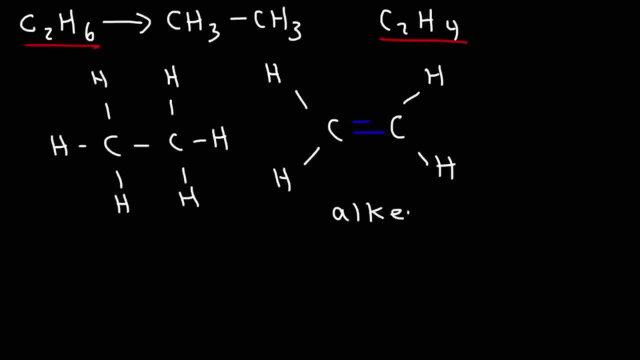 And so this is known as an alkene. Alkenes contain at least one double bond. Alkenes do not contain double bonds, So a two carbon alkene is known as ethene. Now what about this one, C2H2?? 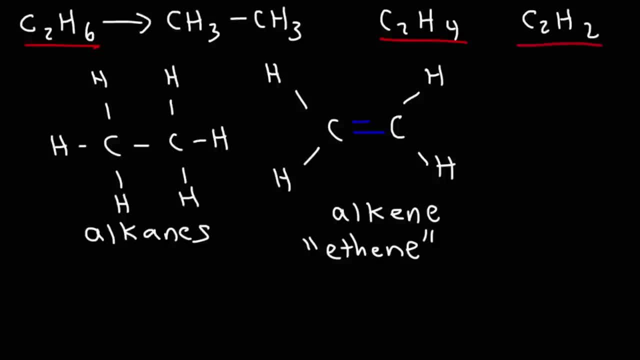 How can we draw the Lewis structure for that? Well, we have a total of two hydrogen atoms, So we're going to put one hydrogen atom on each carbon, And in order for the two carbon atoms to have four bonds, we need to put a triple bond in the middle. 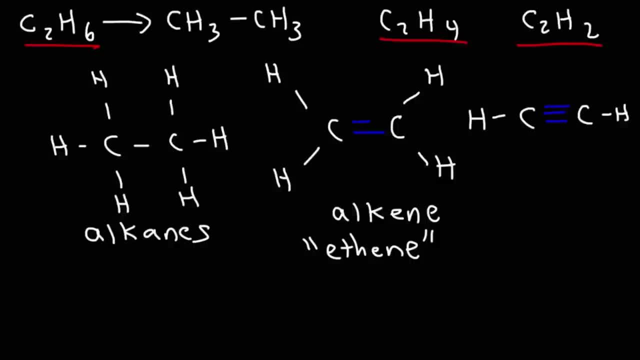 Because carbon likes to form four bonds, And so whenever you have a hydrocarbon with a triple bond, you now have what is known as an alkyne, A two carbon alkyne is known as ethene. The common name for this is acetylene. 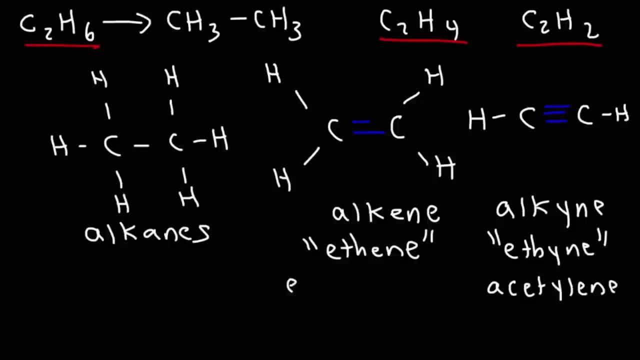 And the common name for this compound is known as ethylene. Alkenes and alkynes are known as unsaturated compounds Because they don't contain the maximum number of hydrogen atoms per carbon atom. Alkenes are known as saturated compounds, So make sure you keep this in mind. 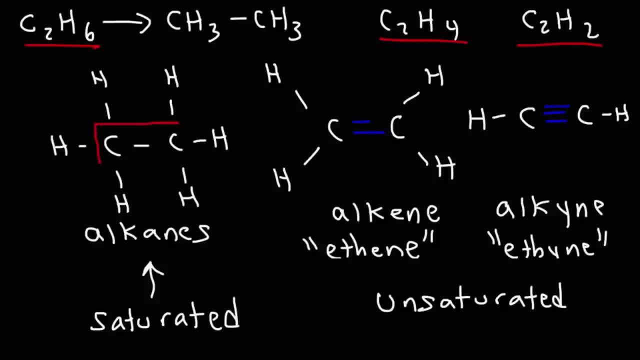 Now let's focus on the carbon-carbon bonds. What would you say? which of these bonds is the longest bond? The carbon-carbon single bond, The double bond Or the carbon-carbon triple bond? Which one is the longest And which one is the shortest? 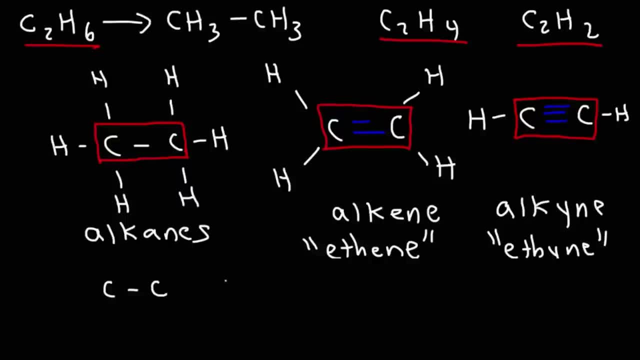 You need to know that the carbon-carbon single bond is longer than the carbon-carbon double bond And that's longer than the carbon-carbon triple bond. The length of the carbon-carbon single bond is 154 picometers, Which is 1.54 angstroms. 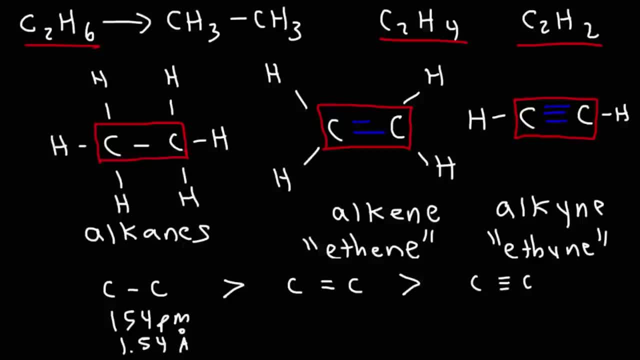 1 angstrom is 100 picometers. The CC double bond is 133 picometers. in ethene- And in ethine- I mean ethine- it's 120.. So what you need to understand is that triple bonds are short bonds. 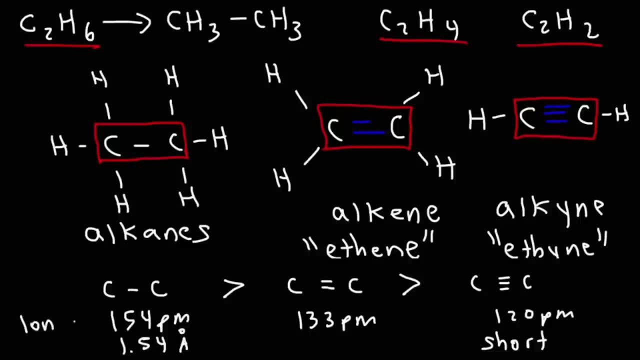 Whereas single bonds are long bonds Because sometimes you may get a test question that asks you something about bond length: Which of these bonds is the shortest Or which of these bonds is the longest? So single bonds are longer than triple bonds. Keep that in mind. 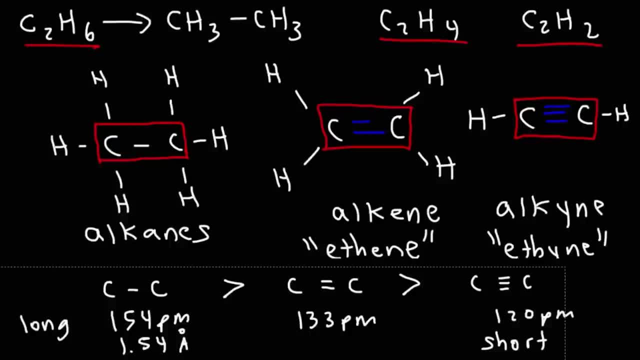 So now that we've talked about bond length, let's talk about bond strength. Which bond is the strongest, The single bond, The double bond Or the triple bond? What would you say? The single bond is the weakest, The triple bond is the strongest? 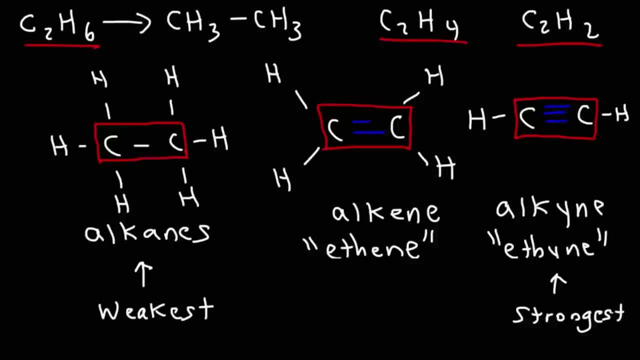 Why is that? Well, it's easier to break one bond instead of three bonds. Imagine trying to break a pencil. It's easier breaking one pencil than trying to break three pencils at a time. Three bonds are stronger than one. Now let's talk about sigma and pi bonds. 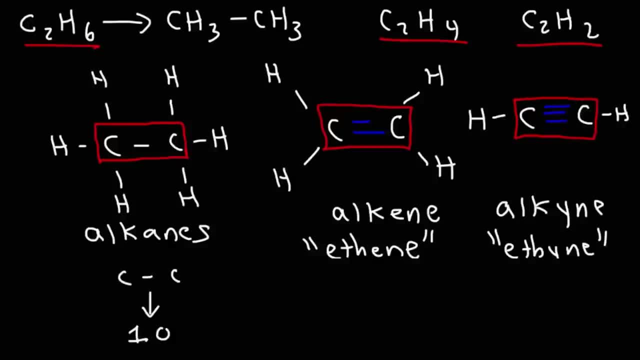 A single bond contains one sigma bond. All single bonds are sigma bonds. A double bond contains one sigma and one pi bond. The triple bond contains one sigma and two pi bonds. Now, which bond is stronger, A sigma bond or a pi bond? 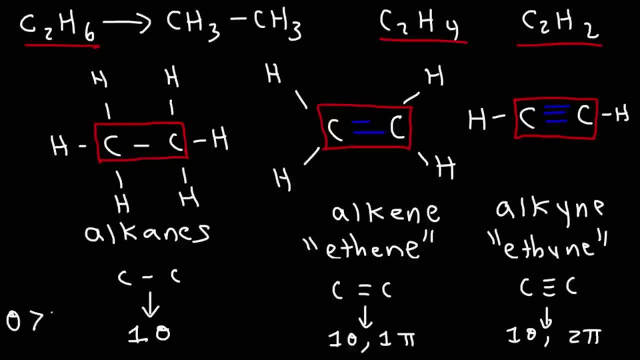 You need to know that sigma bonds are stronger than pi bonds, So it's harder to break this bond versus just one of the pi bonds in the triple bond. Not all three bonds, but one of the pi bonds. So, in summary, a triple bond is stronger than a single bond. Because you're comparing three bonds to one. However, a sigma bond is stronger than a pi bond when you're comparing one bond with one bond. So I'm just going to say that one more time: Sigma bonds are stronger than pi bonds, but triple bonds are stronger. 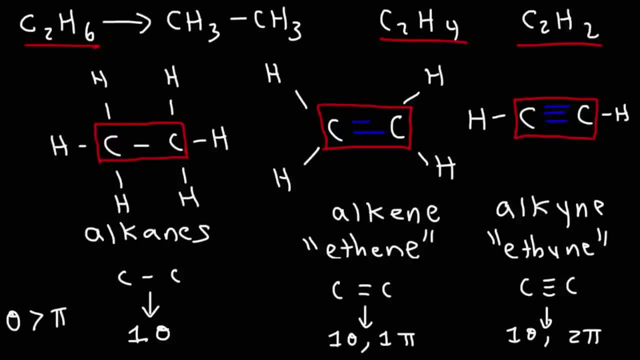 than single bonds. Now the next thing we're going to talk about is bond order. What is the bond order for a single bond, a double bond and a triple bond? This one is pretty straightforward: For a single bond, the bond order is one. 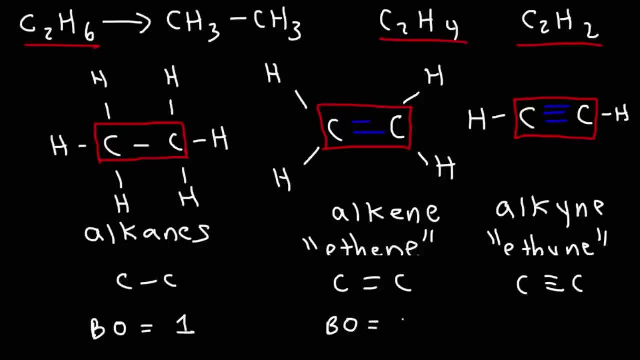 For a double bond, the bond order is two, And for a triple bond, the bond order is three. So that's just something to know. Now let's talk about hybridization. What is the hybridization of the carbon atoms highlighted in green? 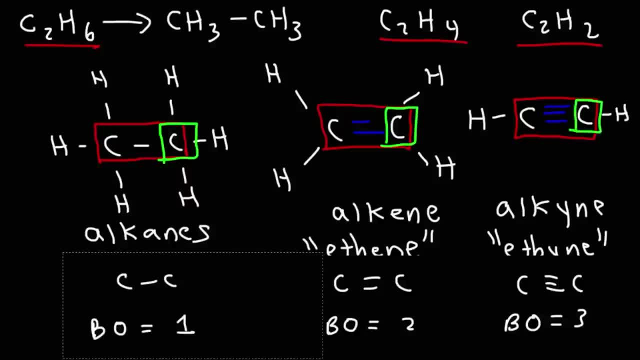 Would you say it's S, sp2, sp3, sp, dsp3,, d2sp3?. What would you say? A quick and simple way to determine the hybridization around a certain carbon atom is to count the number of atoms attached to that particular carbon atom. 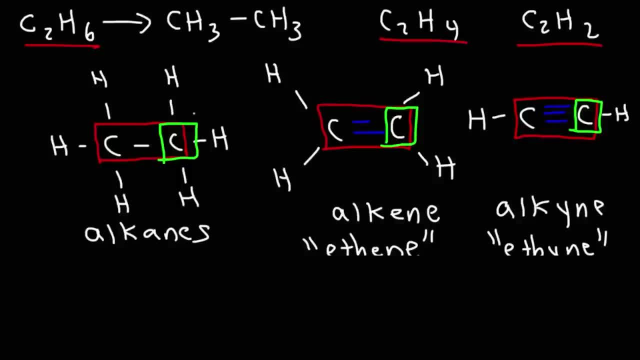 and the number of lone pairs that it has. So this particular carbon atom is attached to four other carbon atoms, So you could think of it as having four groups around it. So the hybridization is going to be S1p3, because the exponents add up to four. 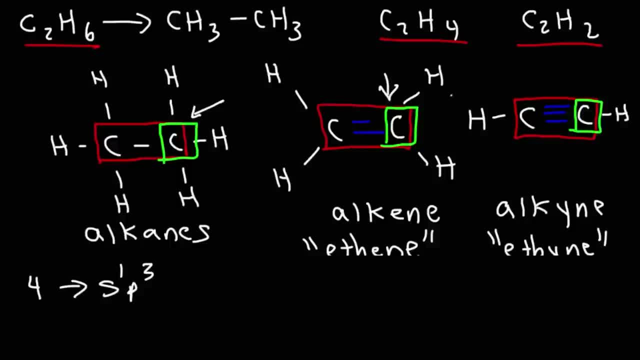 Now let's say, if we want to determine the hybridization of this carbon atom, That carbon is attached to three other atoms, So it has three groups around it. The hybridization is going to be S1p2 or sp2 hybridized. 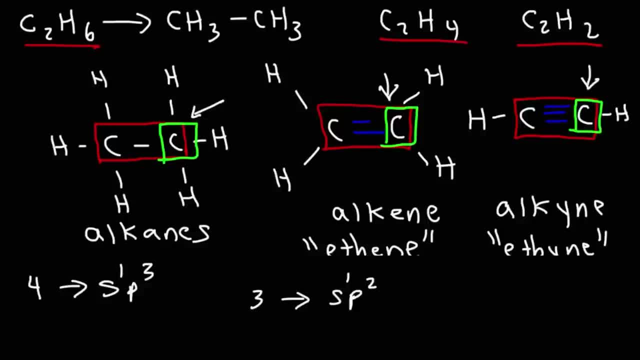 And then for this particular alkyne, the carbon atom has two atoms attached to it, So for two groups it's going to be sp hybridized. So that's a quick and simple way to determine the hybridization of a carbon atom. 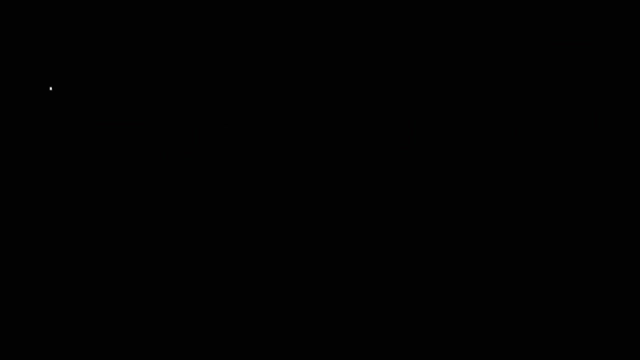 Here's a question for you. So let's say we have a Lewis structure that looks like this: What is the hybridization of? not the atoms, but the bond. What is the hybridization of the CH bond and also of this particular CH bond? 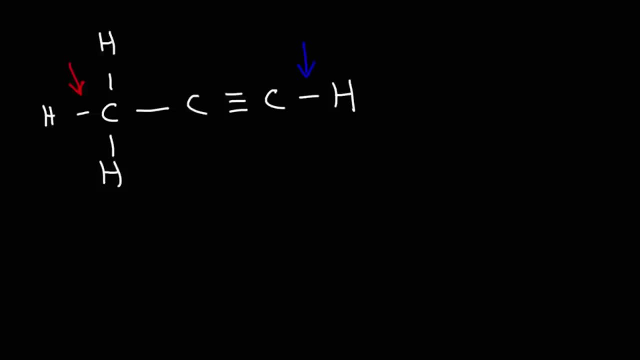 What would you say If you were to get a test question that asks you that question? how would you determine the hybridizations of this bond highlighted in red and this bond highlighted in blue? What you need to do is determine the hybridization of the atoms. 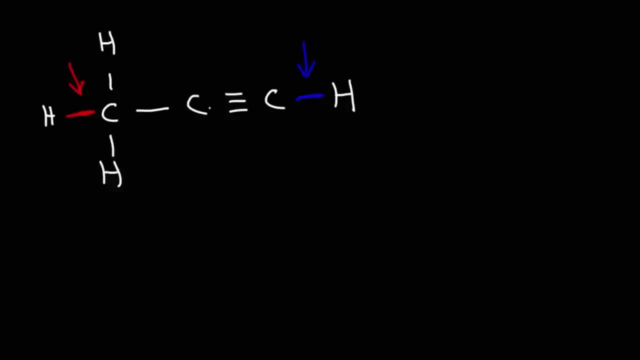 that are connected to those bonds. So what is the hybridization of this carbon atom? That carbon is attached to four other atoms, So it has four groups, and so it's going to be sp3 hybridized. Now you need to look at the other atom, the hydrogen. 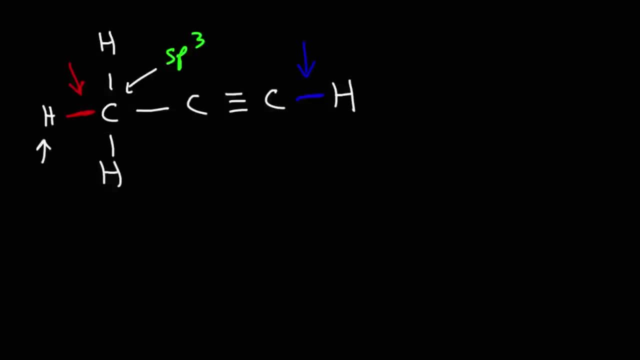 Hydrogen is only attached to one atom. So what do you think the hybridization of hydrogen is going to be? This is going to be S. So that's the hybridization of the CH bond. That's going to be sp3-S. 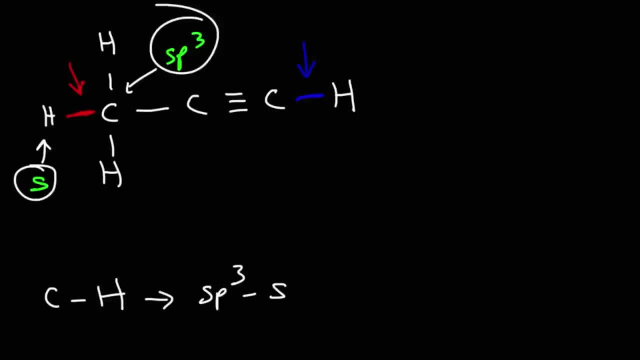 You simply just write both of these together. Now, what about the CH bond highlighted in blue? What is the hybridization of that CH bond? Feel free to pause the video If you want to try it. So let's start with the carbon atom. 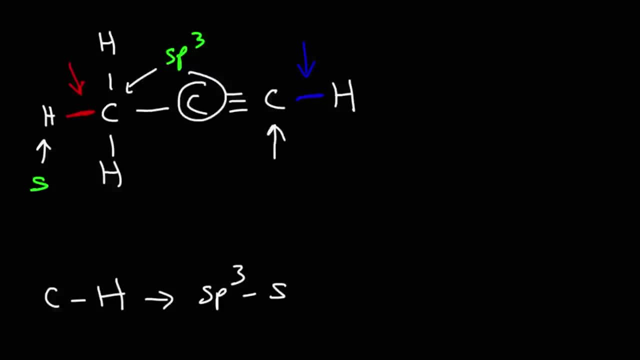 That carbon is attached to two other atoms, So it's going to be sp hybridized, and hydrogen is always S hybridized, So that particular CH bond is going to be sp-S hybridized. Now another question that you might be asked, given this: 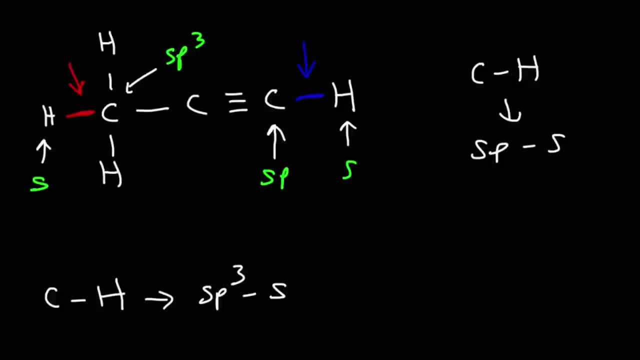 this compound is how many sigma and pi bonds are in this compound? Feel free to pause the video and try it. So first let's count the number of sigma bonds. Every single bond is a sigma bond. So we have one, two, three. 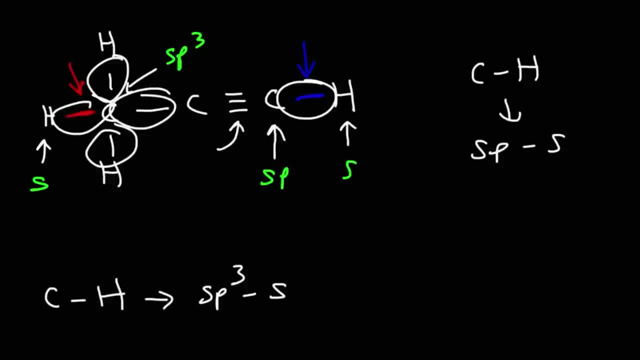 four, five And there's one sigma bond in the triple bond. So we have a total of six sigma bonds. Now, how many pi bonds do we have? We know that a double bond contains one pi bond. A triple bond contains two pi bonds. 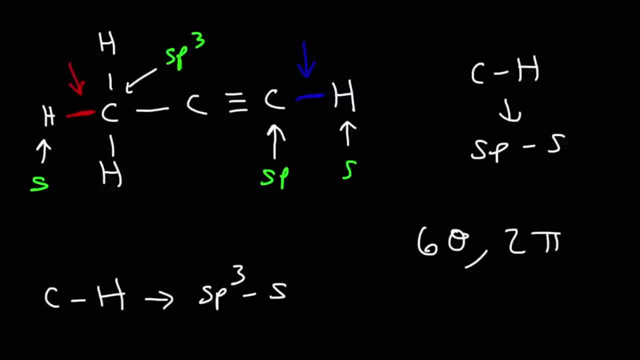 So this molecule have six sigma bonds and two pi bonds. So that's how you could determine the number of sigma and pi bonds in an organic compound. Now the next topic of discussion is how to calculate the formal charge of an element. So let's use carbon as an example. 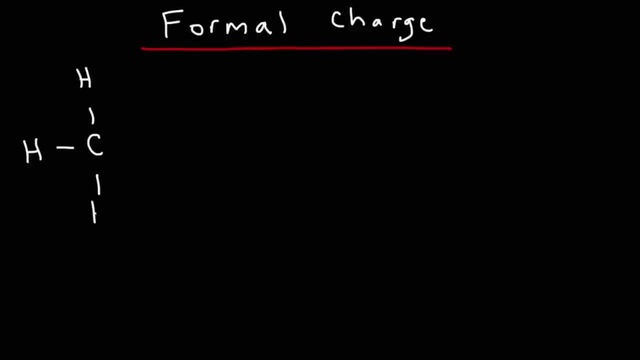 Calculate the formal charge of each carbon atom for these three situations. If you know how to do it, feel free to go ahead and try it. Now. there's a formula that will help you to calculate the formal charge of an atom, And here it is. 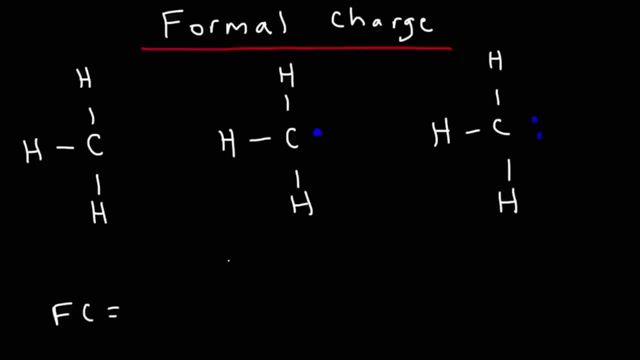 The formal charge is going to be equal to the number of valence electrons of the element, minus the number of bonds and dots attached to that element. So for the first example, carbon has four bonds. I mean, let me say it again, Carbon has four valence electrons. 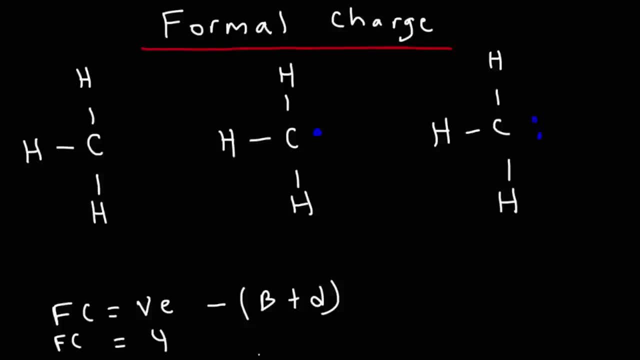 It's in group 4A of the periodic table And in this example it has three bonds: one, two, three, and it doesn't have any dots around it. So four minus three is one. So this particular carbon atom has a formal charge of plus one. 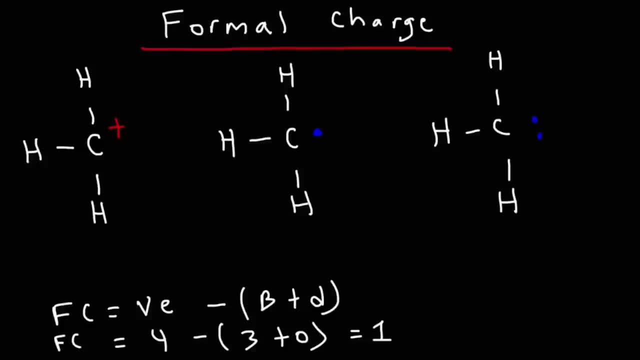 So we could say that it has a positive formal charge. Now, moving on to the next one, it's going to be four valence electrons minus three bonds and one dot. So we got three bonds and one dot, That's four minus four. 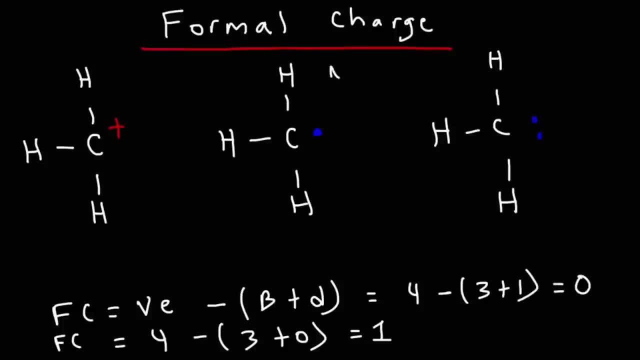 So that's zero. So this one is neutral. It doesn't have a charge. Now for the last example on the right, the valence electrons of carbon will still be the same. We still have three bonds, but this time we have two dots. 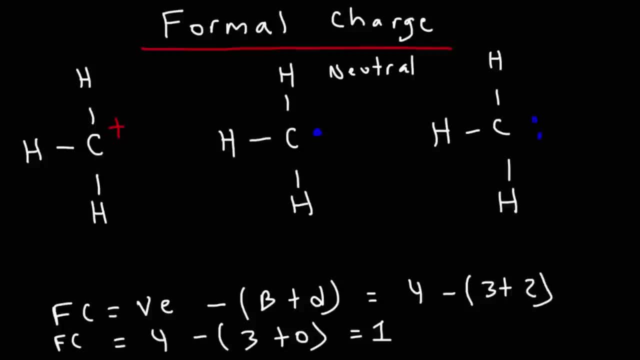 One lone pair is equivalent to two dots. So three plus two is five. Four minus five is negative one. So this particular carbon atom has a negative charge. We said that positive. Let me say that again. We said that positively charged ions are called cations. 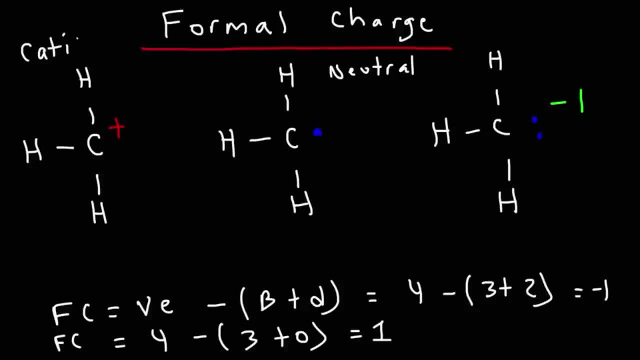 and negatively charged ions are known as anion. When you add a carbon to it, this is called a carbocation, And on the right, this is called a carbanion- Carbanion Carbanions have negative charges. Now, when you have an odd number of electrons, 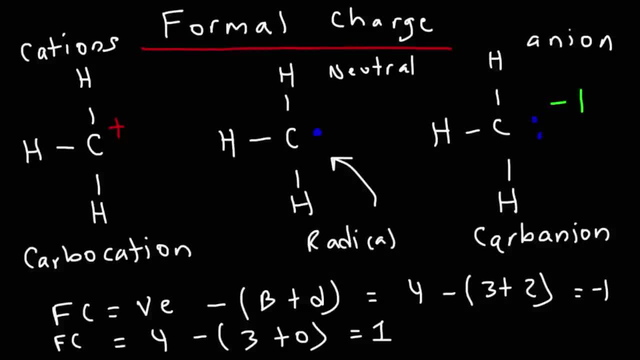 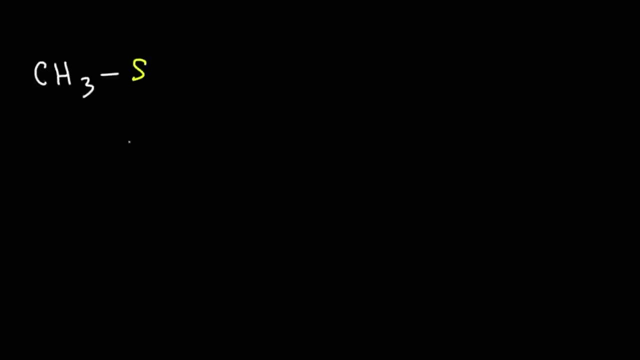 you have what is known as a radical. So a one-carbon radical is known as a methyl radical. Radicals tend to be neutral. Now let's work on some more examples. Go ahead and calculate the formal charge of the sulfur atom and also calculate the formal charge. 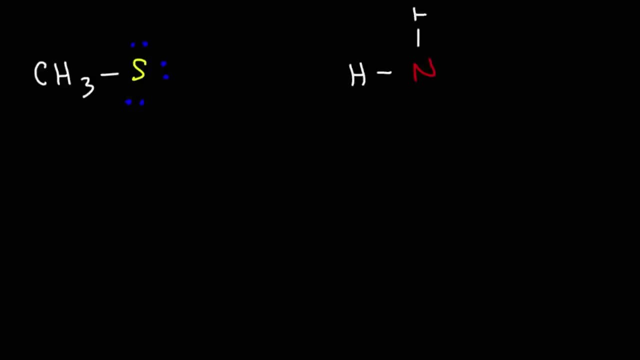 of the nitrogen atom. Go ahead and take a minute to work on that example, Or those two examples, rather. By the way, for those of you who are looking for a specific topic but for some reason you're not finding it in this video, 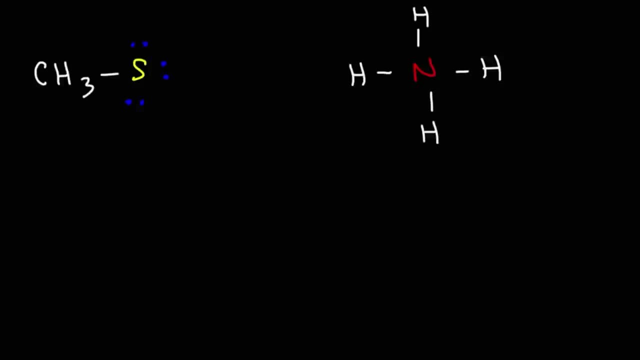 when you get a chance, do a YouTube search, Type in organic chemistry playlists. I have two playlists, an older one and a newer one. The newer one is going to be more helpful, So in that playlist chances are you could find a topic. 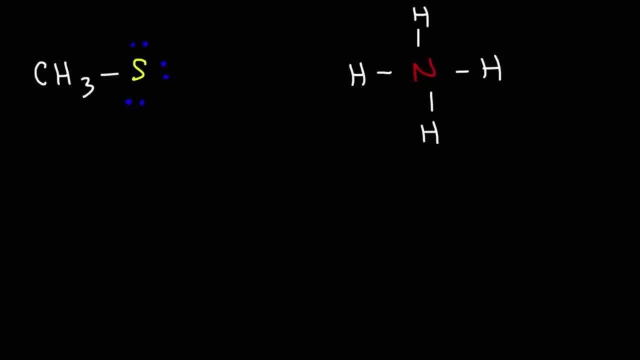 that you might be looking for, So just feel free to take a look at that as well. I'll be posting some links in the description section below this video with some other topics that might help you with the first exam that you might be taking in organic chemistry. 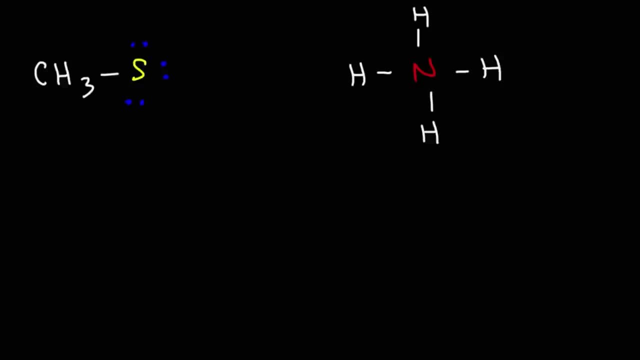 So feel free to check that out as well. So let's begin. Let's start with sulfur. Let's write the formula. So the formal charge is going to be the number of valence electrons minus the sum of the bonds and dots around that element. 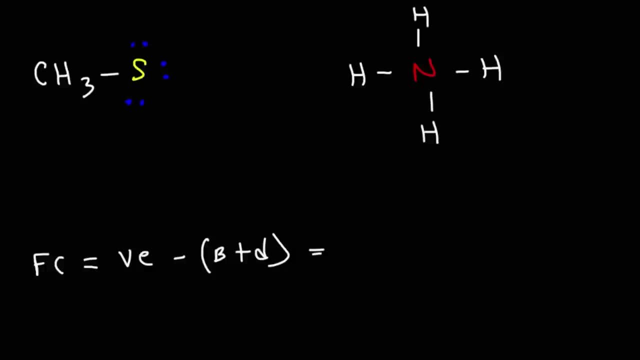 Now, how many valence electrons does sulfur have? Sulfur is found in group 6A of the periodic table. If you don't have one, you could do a Google search. You could find it in Google Images and then you could pull up the periodic table. 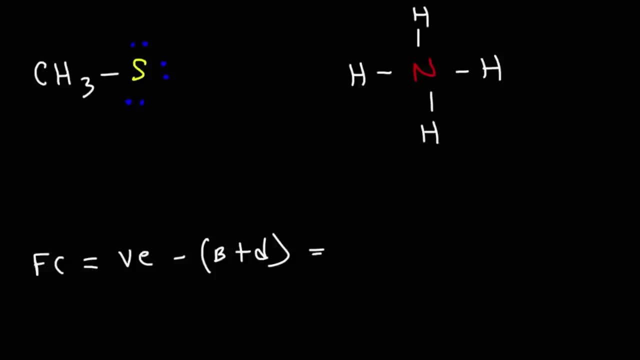 If you look for sulfur, it's right under oxygen And it's in group 6A, which means that sulfur has six valence electrons In this structure. it only has one bond attached to it. Now, how many dots does it have? 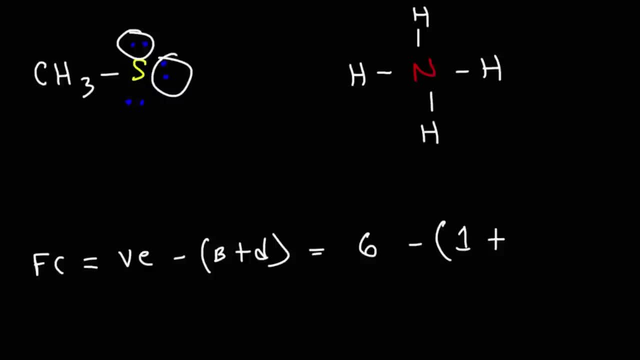 Well, we have three lone pairs, which is equivalent to six dots. So this is six minus seven. So the sulfur atom has a negative one formal charge. Now for nitrogen in the ammonium ion. nitrogen has five valence electrons. It's in group 5A. 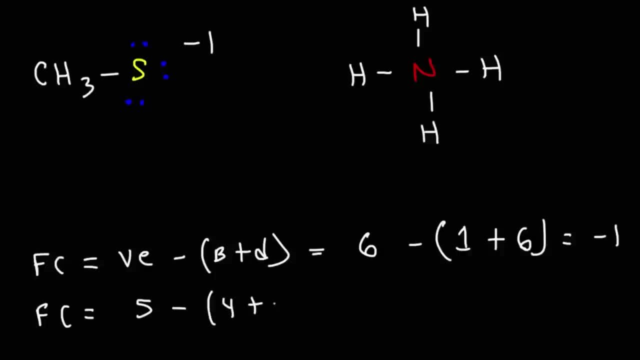 of the periodic table. In this structure it has four bonds, no dots, So five minus four is one. So this particular nitrogen atom has a plus one, or some may say a one plus formal charge. So that's how you could determine the formal charge of an element. 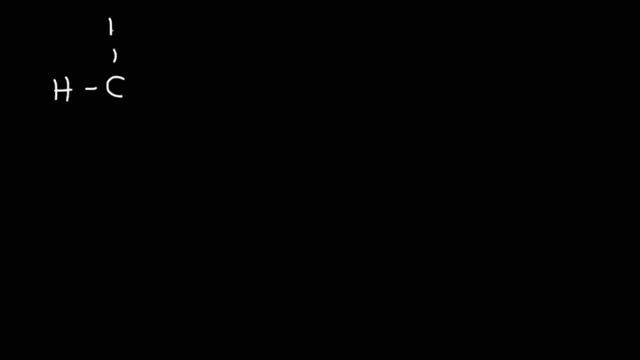 Now let's go back to this structure, because there's another question that I'm going to ask that teaches another concept: How many bonding electrons and nonbonding electrons are present in this ion? What would you say? A lone pair represents a pair of nonbonding electrons. 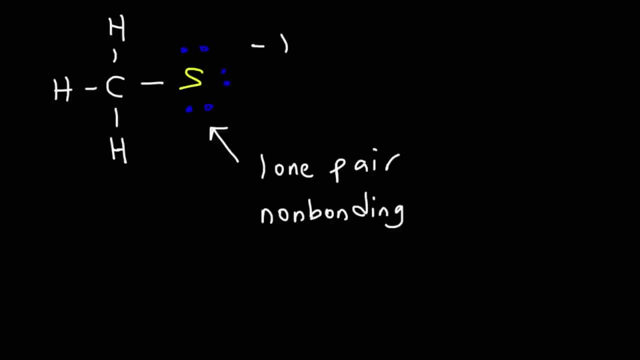 because they're only attached to one atom, So they're nonbonding electrons. In a bond you have two bonding electrons. So to count the number of bonding electrons, this is going to be two, four, six, eight, So this particular ion. 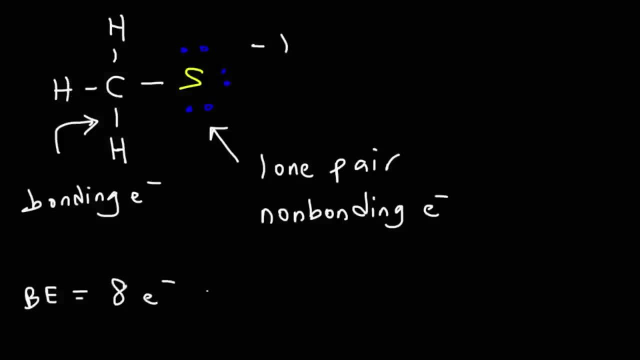 has a total of eight bonding electrons because it has four bonds. Each bond contains two bonding electrons. Now, how many nonbonding electrons do we have? Two, four, six. There's a total of six nonbonding electrons, which equates to three lone pairs. 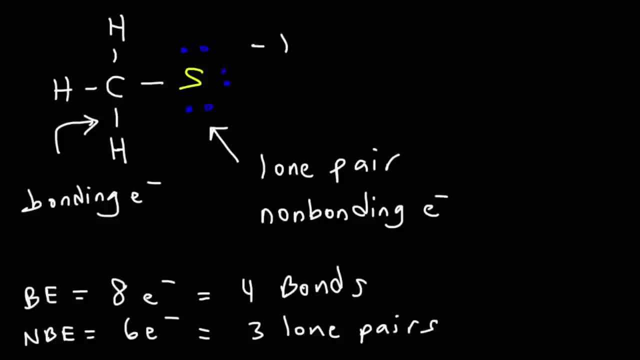 So make sure you understand that concept. One lone pair is equal to two nonbonding electrons, And one bond equates to two bonding electrons. Now let's continue our discussion of drawing the Lewis structures of organic compounds, as well as considering the functional groups. 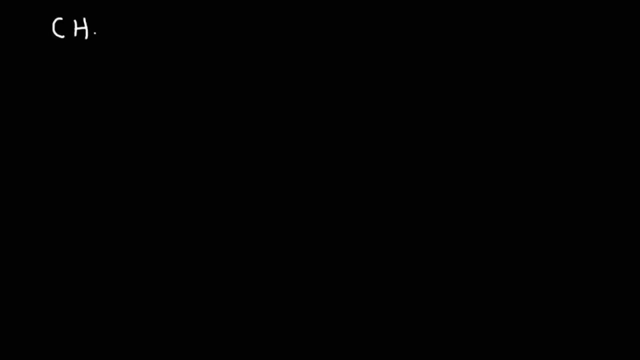 of those compounds. So let's consider CH3CH2OH And let's compare that with CH3CH2OH. So feel free to pause the video and go ahead and draw the two Lewis structures. So for the one on the left. 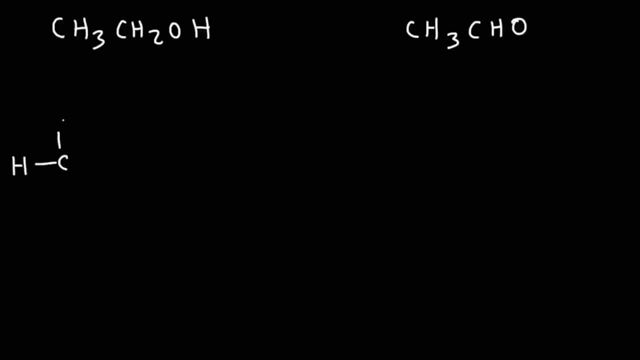 we have a carbon that is connected to three hydrogen atoms And then it's attached to a CH2, that is, a carbon with two hydrogen atoms And that's connected to an OH group. Keep in mind, oxygen likes to have two bonds And it's going to have two lone pairs. 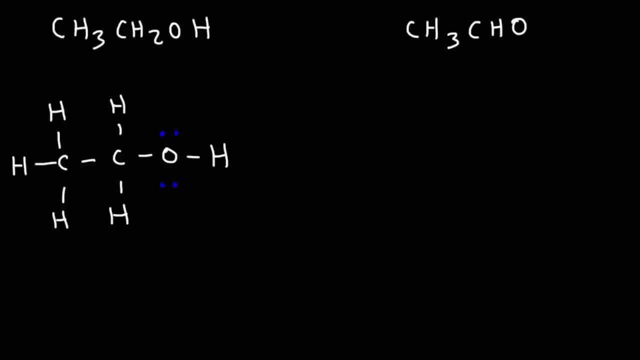 So that's the Lewis structure for this molecule. Now, whenever you see an OH group, this is the functional group of an alcohol And the fact that we have two carbons. this is associated with the alkane ethane. But because we have an alcohol, 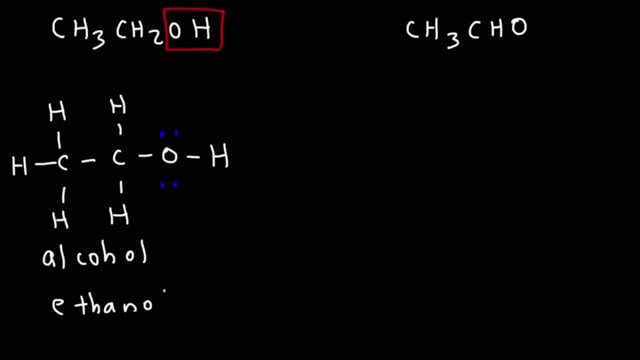 we can name it ethanol, So alcohols have the suffix OL. So this is ethanol. Now what about the structure on the right? So we have a methyl group that is a CH3. And that is attached to a carbon atom. Now it's CHO instead of OH. 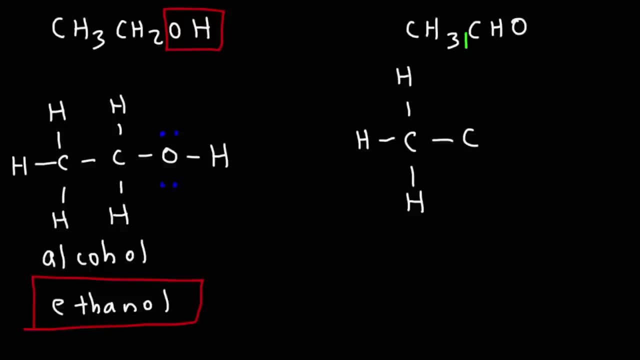 When you see CHO, this is the functional group of an aldehyde. If we were to write OH, this is not going to work because carbon doesn't have four bonds. So that tells you that we need a different structure. An aldehyde contains a carbonyl group. 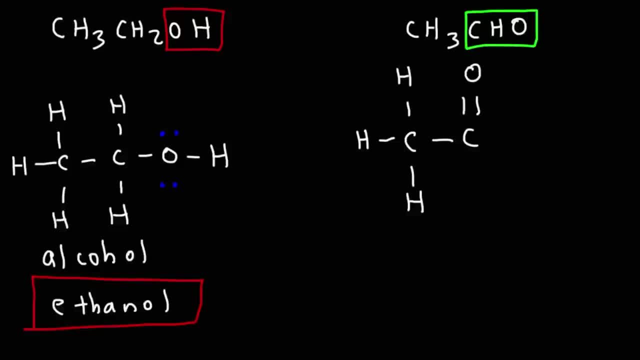 Which is basically a carbon double bonded to an oxygen, And then here's the hydrogen. So in this case, every carbon atom has four bonds, Every hydrogen atom has one bond And the oxygen atom has two bonds, Which is what they usually have. 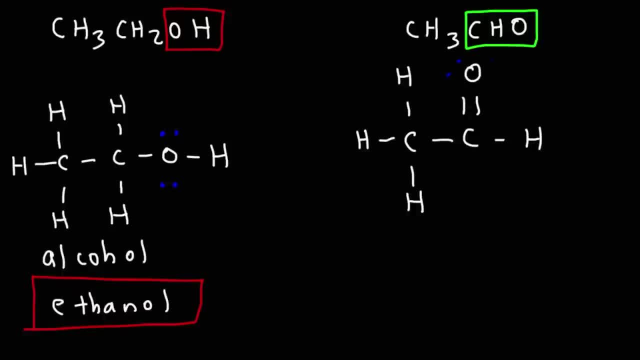 in neutral molecules And, of course, the oxygen is going to have two lone pairs, as it did here. So this is a carbonyl And this particular carbonyl which is attached to a hydrogen that is known as an aldehyde. 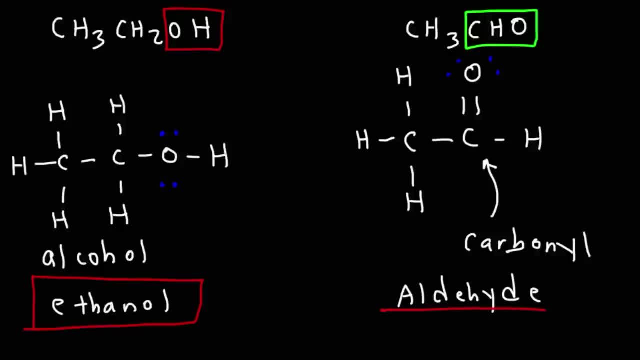 So that's the name of the functional group. A two carbon aldehyde is called ethanol Instead of ethanol, So it ends in AL as opposed to OL. The common name for this aldehyde is acetaldehyde. Now let's consider these two examples. 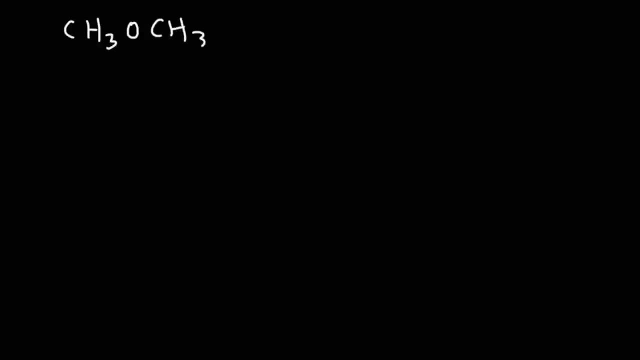 CH3OCH3 and CH3COCH3.. Notice the difference? So go ahead and draw the Lewis structure for these two organic compounds. For the first one, we have a methyl group, That's a carbon with three hydrogen atoms, And then we have an oxygen in the middle. 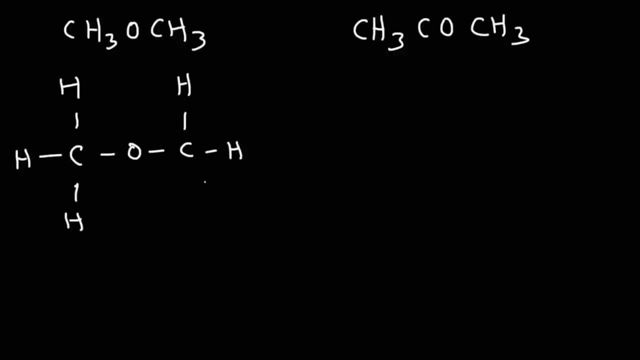 As we said before, oxygen likes to form two bonds And then another methyl group to the right of that. So this particular compound has a functional group known as an ether. An ether is basically an oxygen atom between two carbon atoms. That's an ether. 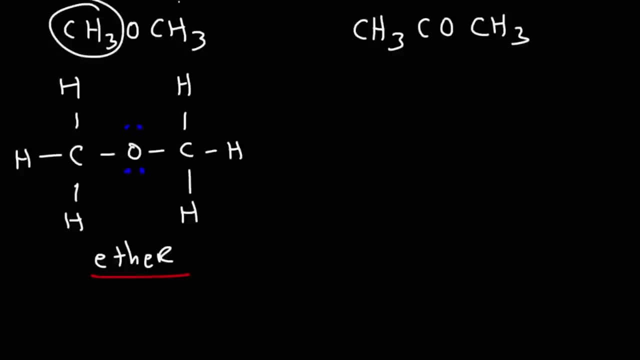 Now, because this particular ether has two methyl groups, one to the left, one to the right. this is known as a dimethyl ether. The prefix di- means two, Tri- means three, Tetra- means four, Penta- means five. 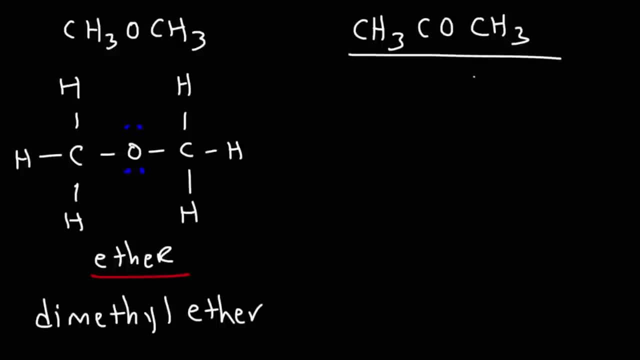 Now, how would you draw the Lewis structure for the compound on the right? So we know that we have a methyl group on the left And then there's a carbon atom. Now where do we put the oxygen atom If we put it in the middle? 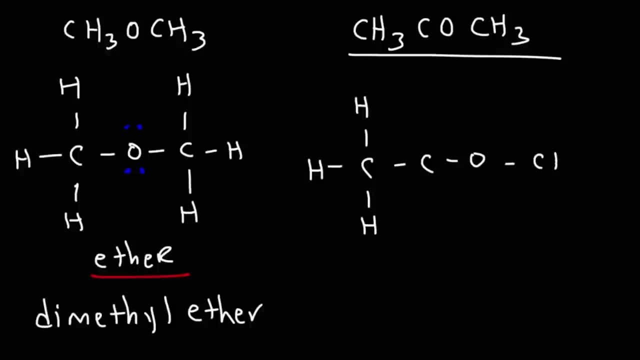 this carbon atom is going to have two bonds. So to fix that problem- we need to put it up here- We need to make another carbonyl functional group And then write the methyl group. So in this case every carbon atom has four bonds. 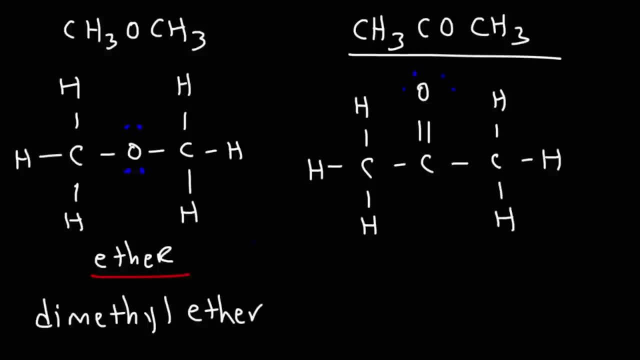 The oxygen atom has two bonds And every hydrogen atom has one bond. That's why it's important to know the number of bonds each element like to make, because it makes drawing the Lewis structures a lot easier. Now, even though we have a carbonyl, 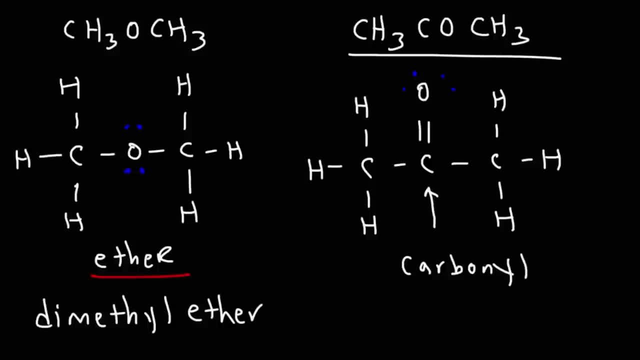 functional group. the name of the functional group for this particular molecule is different than an aldehyde. This is known as a ketone When the carbonyl group is in the middle of the chain. it's a ketone When it's at the end of a chain. 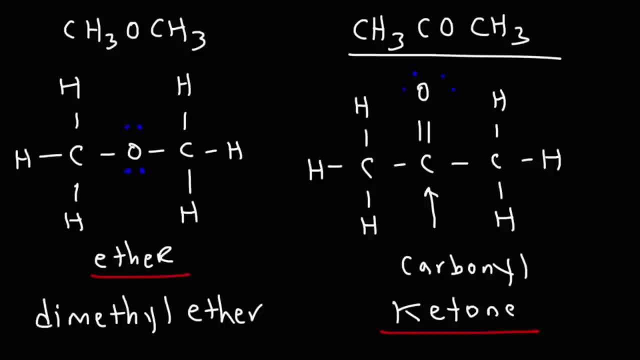 it's an aldehyde. So to name this particular ketone, it's called propanone. Think of propane for a three carbon alkane. So a three carbon ketone is going to be propanone. Ketones have the suffix O-N-E. 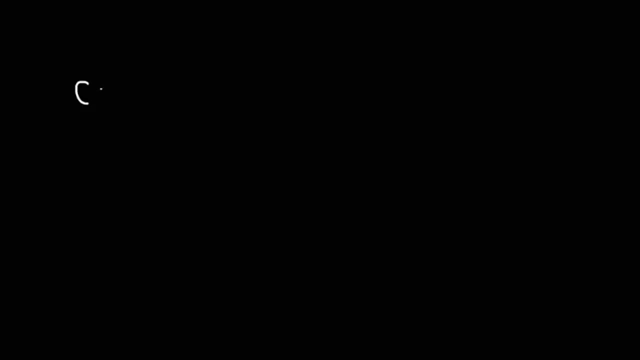 So notice the difference between a ketone and an aldehyde. A ketone will have the carbonyl group in the middle. An aldehyde will have the carbonyl group at the end. So an aldehyde has a hydrogen that's attached to the carbonyl group. 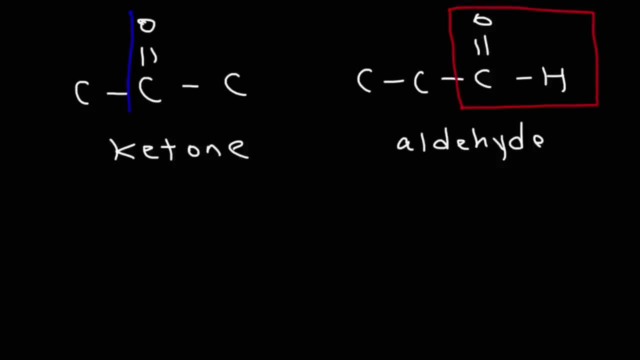 A ketone does not have the hydrogen attached to the carbonyl group, And that's how you can distinguish a ketone from an aldehyde, even though they both have the carbonyl functional group. Now here's the next one: CH3CO2CH3. 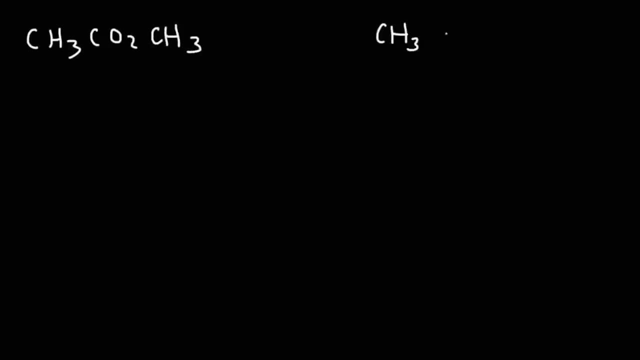 versus CH3 and then CH2 times 3 CO2H. Go ahead and draw the Lewis structures for those two molecules. So I'm not going to completely draw it out, I'm going to expand the condensed structures. So instead of writing C, 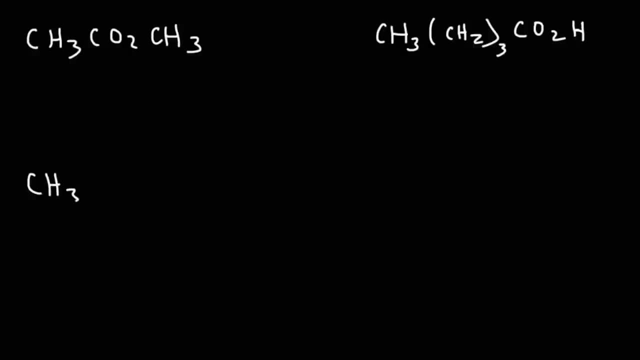 with three hydrogens. I'm going to leave it as CH3. And I'm going to expand this part. It's not going to be like this, because carbon doesn't have four bonds. Instead, the CH3 is going to be attached to a carbon. 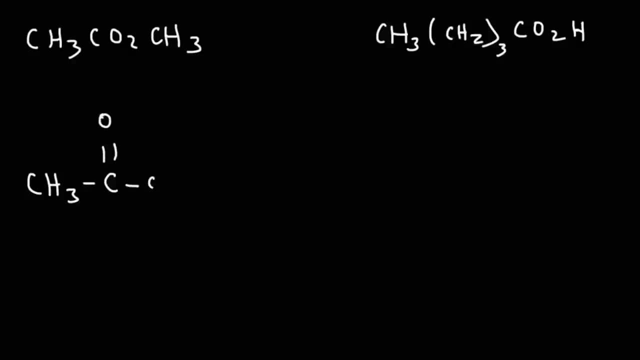 We're going to have a carbonyl group and then an oxygen attached to a CH3. So this functional group is known as an ester. An ester has two oxygen atoms and it has a carbonyl group On the right. 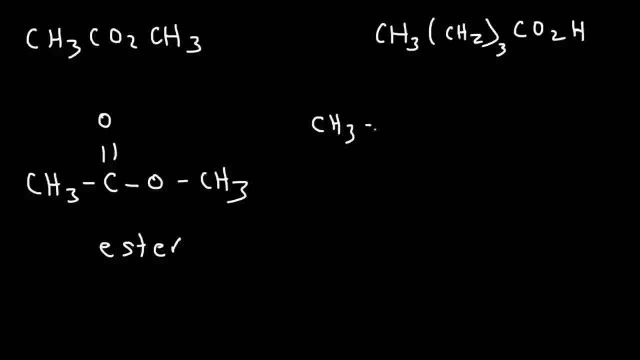 we have a CH3.. That's a methyl group. And then we have three methylene groups, So CH2CH2CH2.. And then we have CO2H, which you can write as COOH, But we're going to expand that further. 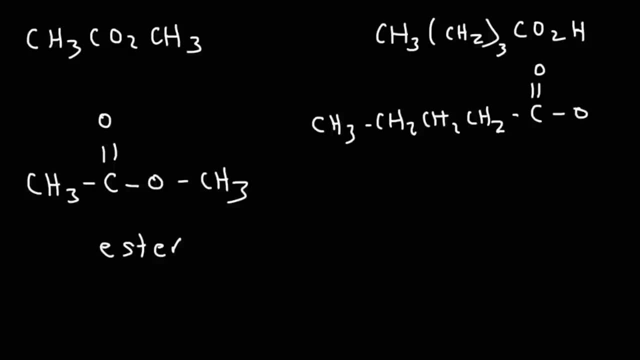 So we're going to have a carbonyl group and a hydroxyl group. So when you combine a carbonyl group and a hydroxyl group, like that, you get a functional group called a carboxylic acid. Now, that particular carboxylic acid. 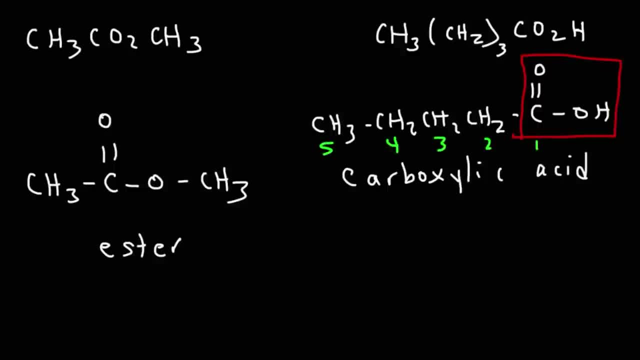 has a total of five carbon atoms. A five carbon alkane is known as hexane, So a five carbon carboxylic acid is going to be called. Wait, let me take that back. A five carbon alkane is not hexane, but pentane. 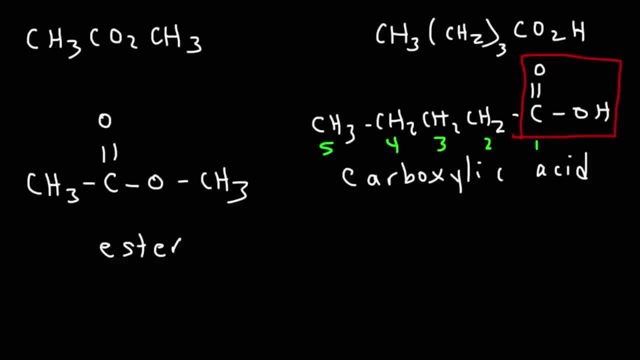 Hexane has six carbons, So a five carbon carboxylic acid is going to be called pentanoic acid, So that's how you can name that particular carboxylic acid. Now, as for the ester, we have a methyl group. 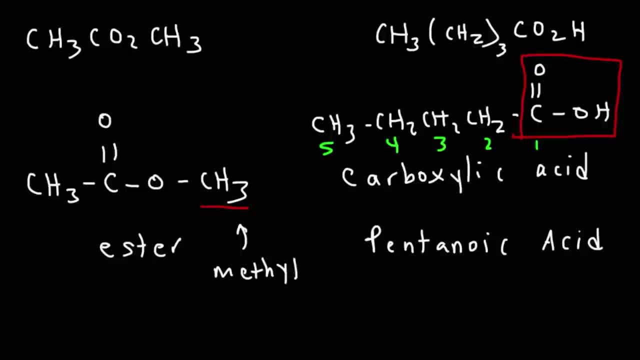 And then here we have a two carbon group with two oxygens, which is called ethanoate. So combined, this is called methyl ethanoate. If you want more examples on how to name esters, just type in ester nomenclature in the YouTube search bar. 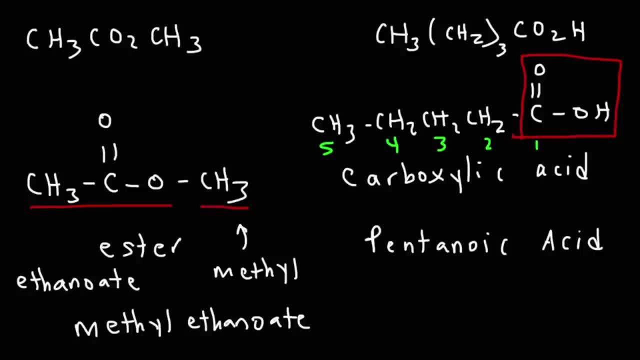 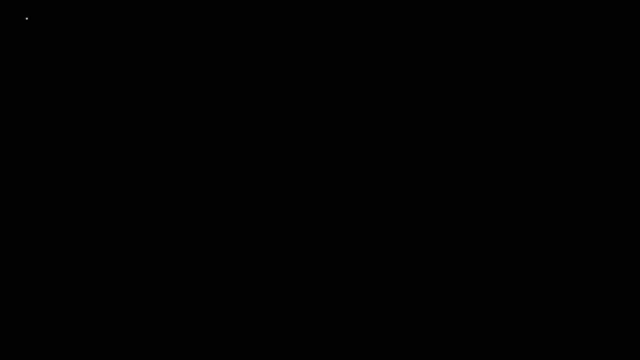 and you'll see some videos come up that has more examples on how to name esters, But that's how you can name this particular one. It's called methyl ethanoate. Now here's a challenge problem. Go ahead and expand this particular structure. 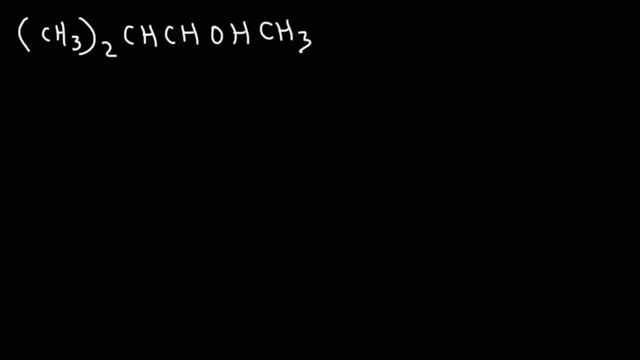 You don't have to worry about naming it, But go ahead and expand it. What I would do is I would start with the CH group there, So we have a carbon attached to a hydrogen, And then that carbon has two methyl groups attached to it. 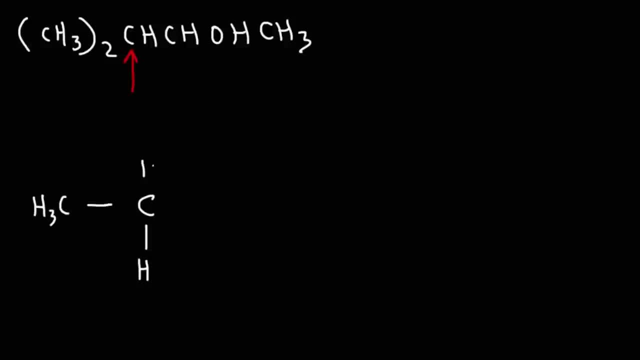 So we have one over here and then another one on top, So this CH is the CH that we see here, And then to the right there is another CH next to it. So I'm going to put carbon with a hydrogen, So that's the CH of this group. 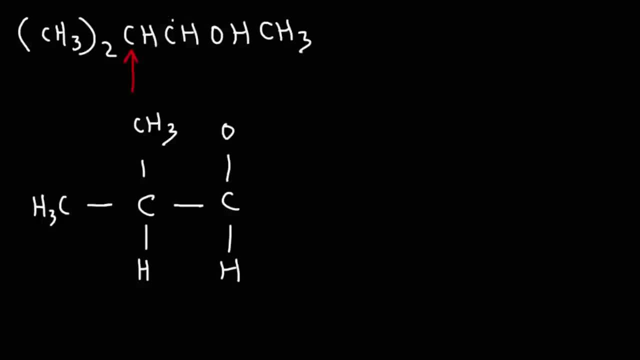 And then attached to that is an OH which we can put here, And then a CH tree, The CH trees or the methyl groups. they're always at the end of a structure, Never in the middle. The CH groups tend to branch out.